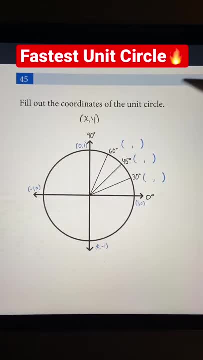 This is the easiest way to memorize the coordinates of the unit circle. Okay, so first thing is: first, what you want to do is you want to do a divided by 2 on each term in the coordinates. Okay, so once you do that, what you want to do is you want to write a 1, 2, 3 down from the left. 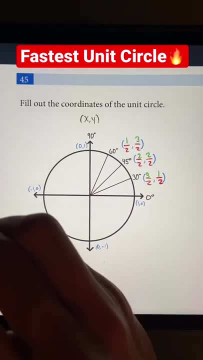 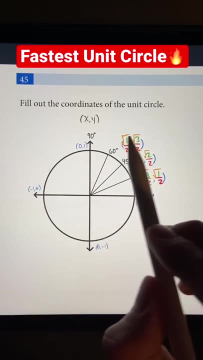 and a 1,, 2,, 3 going up on the right. Okay, so we're almost done. All we have to do is square each of the numerators And once we have that, we know that the square root of 1 is just going to be 1,. 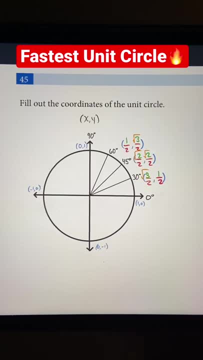 so we can actually remove that square root and we can do the same thing right here And just like that you know the coordinates of the unit circle. 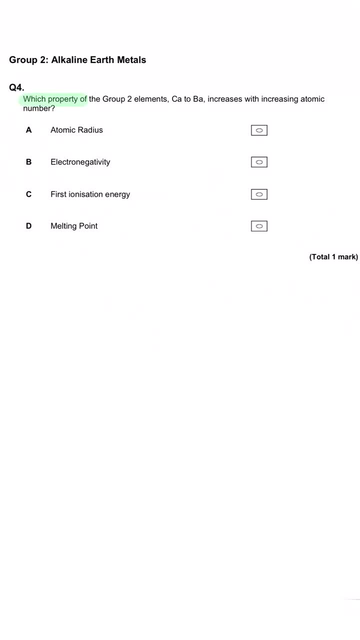 Which property of the group 2 elements, calcium to barium, increases with increasing atomic number, A Atomic radius. This is in fact the correct answer. The atoms have extra energy levels as you work your way down the group, and so the radius of that atom is from the nucleus to the outermost electron, and so this will increase.